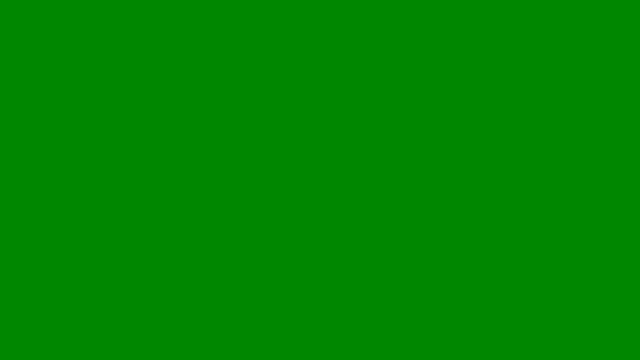 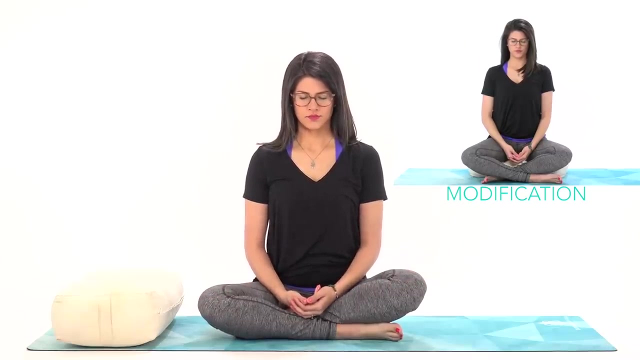 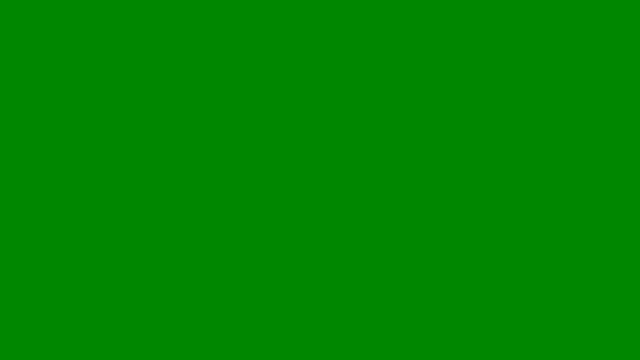 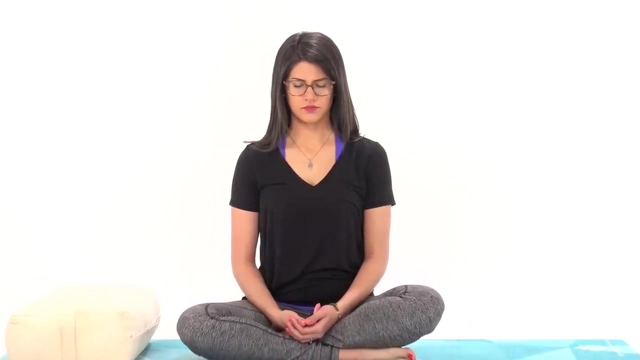 Gently close your eyes And release everything you don't need, as you observe your breath moving in and out through your nose. This is a meditative practice, So once we get into our postures, I'll allow you to just be with minimal to no cues, so that you can find your stillness. 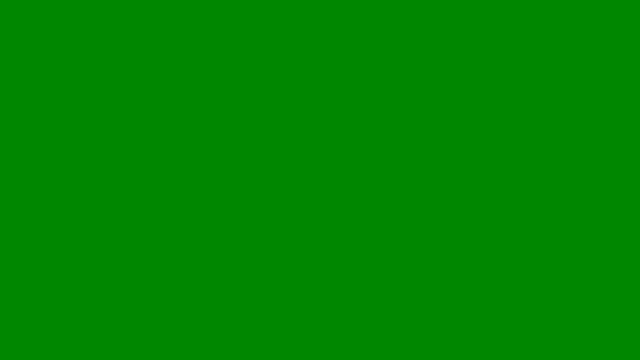 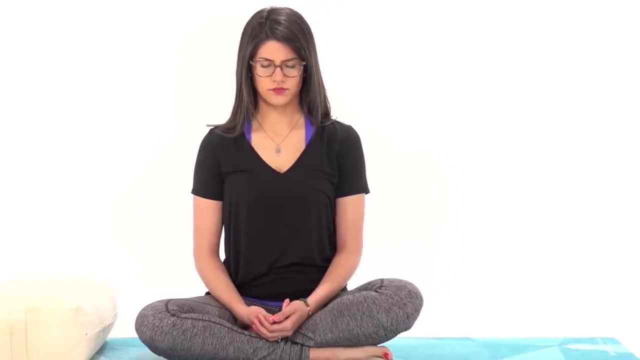 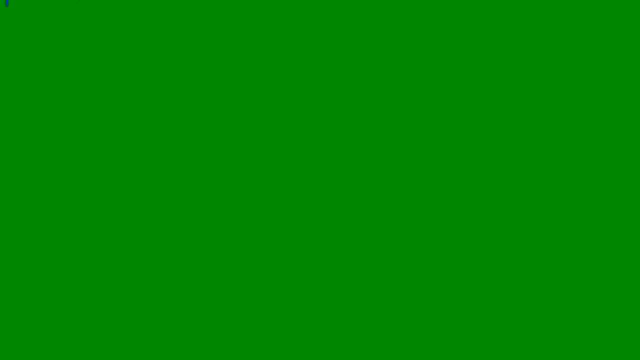 And every time you want to fight or distract yourself, turn your attention back to feeling your deep breath in and out And out through your nose as you relax deeper over time. You're welcome to keep your eyes closed, moving slow, Come to lie down on your back and assist. 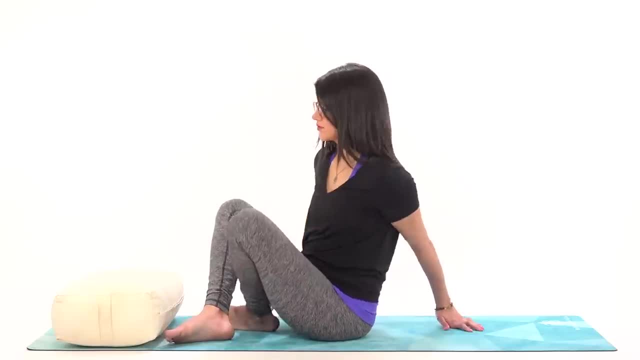 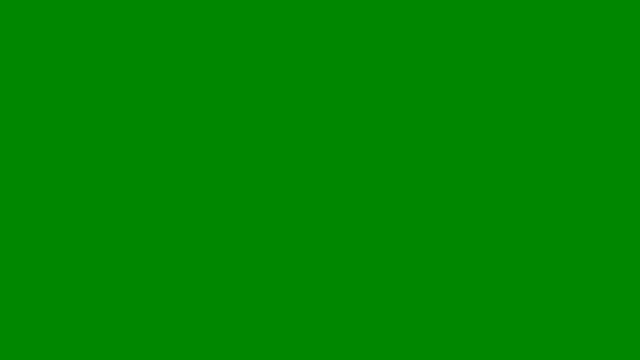 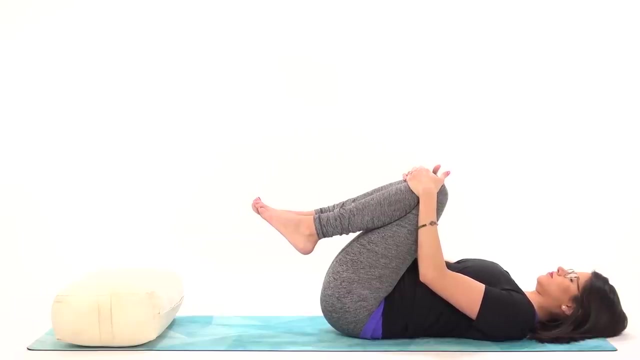 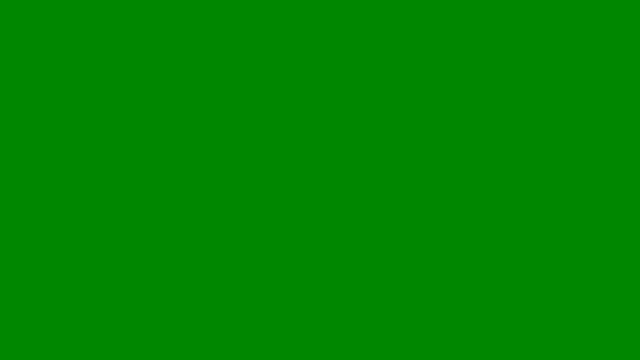 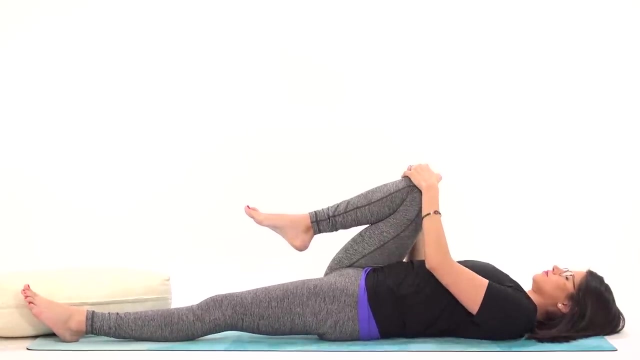 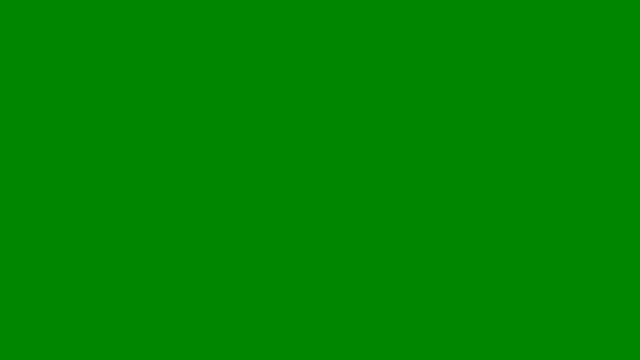 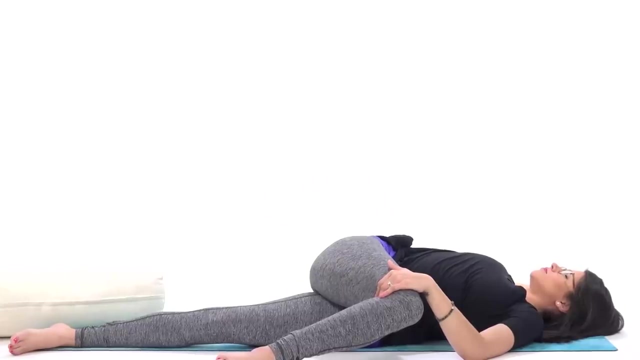 your knees together and into your chest for a full wind pose. Keep your right knee in, Extend your left leg long down on your mat And draw your knee across your body through a supine spinal twist. It's okay if your opposite shoulder peeled up slightly. 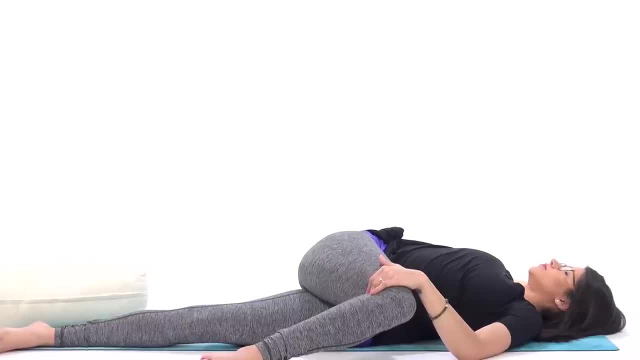 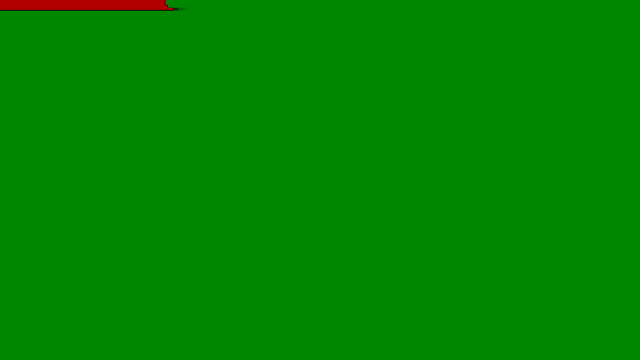 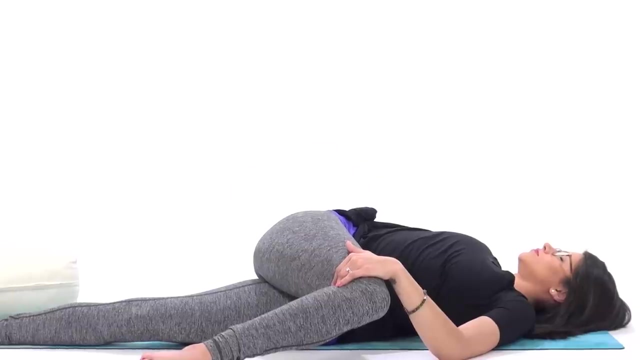 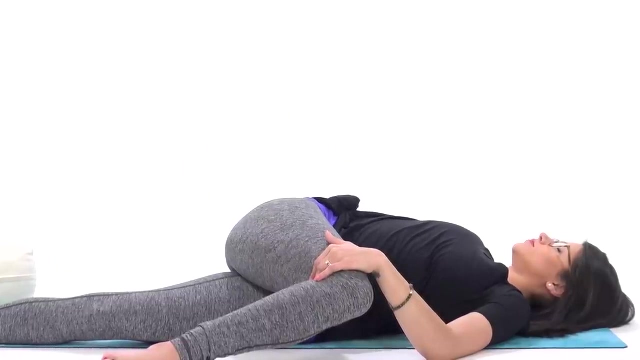 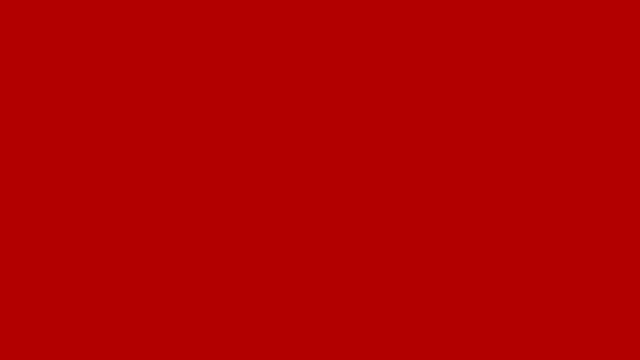 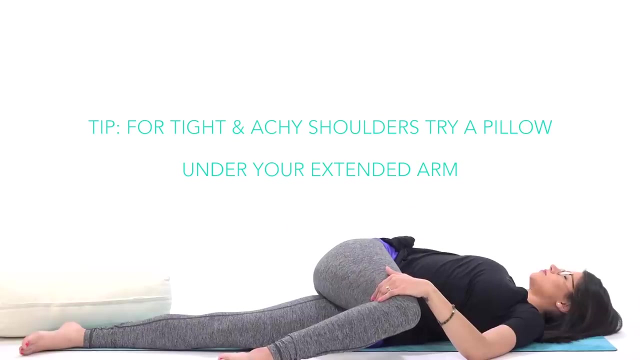 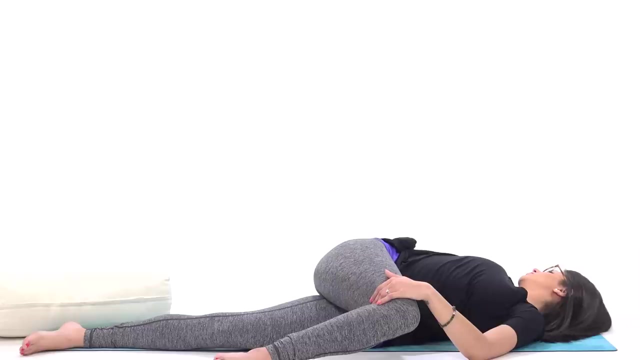 Just breathe, Massaging the muscles in your torso with each and every breath, and trust that your body will relax into place over time. Thank you, Thank you, Notice, if you're holding on to anything unnecessary, Then with each exhale, see if you can let that go. 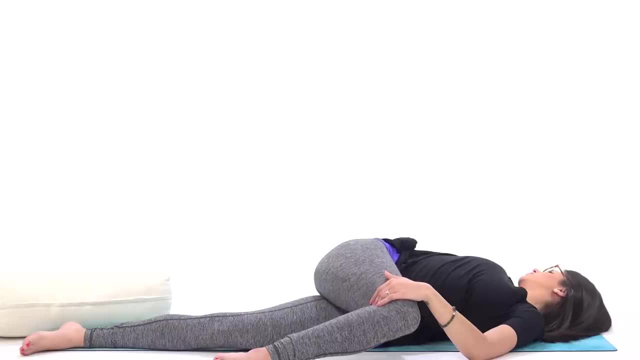 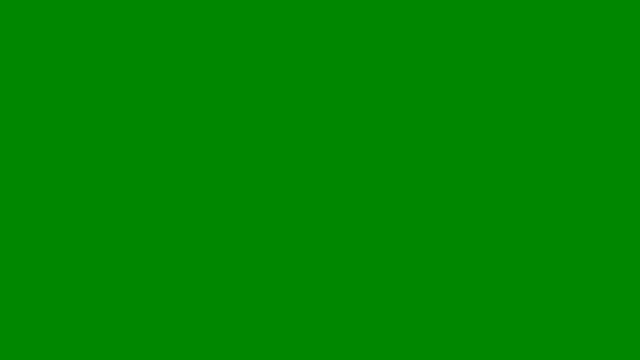 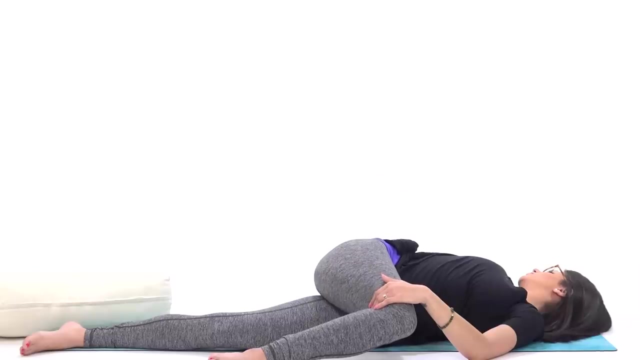 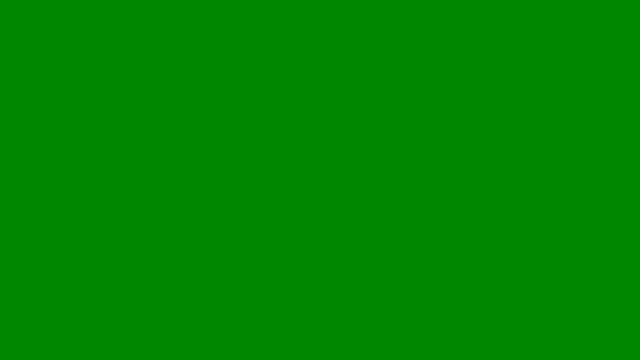 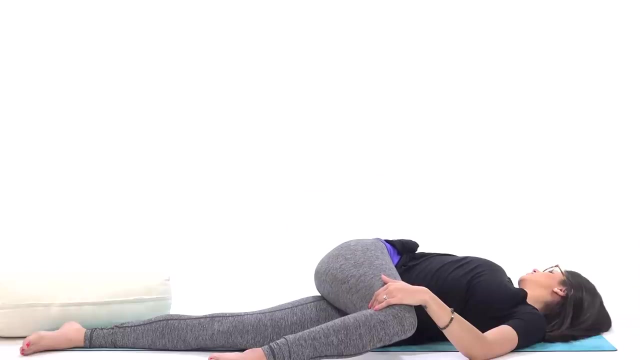 Whether it's physical, in your eyelids or jaw, hands or hips, or mental and emotional thoughts, thought patterns. Find a breath that is cleansing, relaxing and deepening. Slowly undo your twist. Draw both knees into your chest. 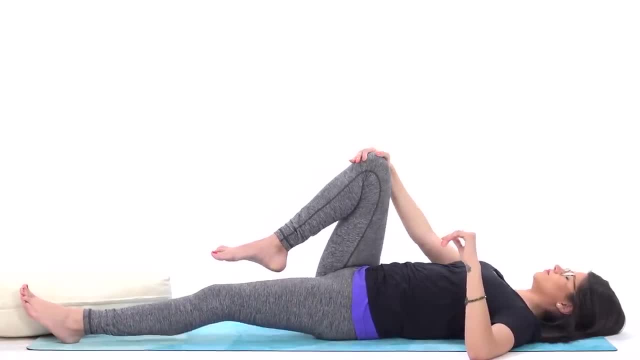 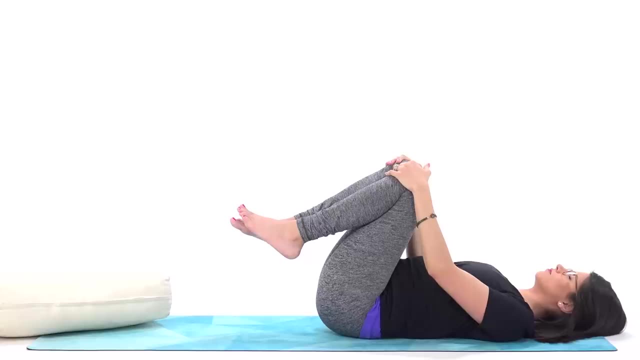 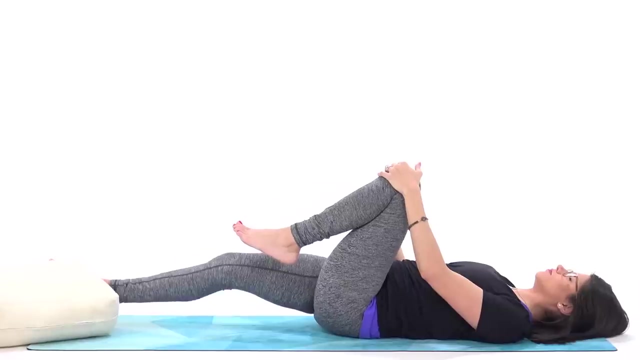 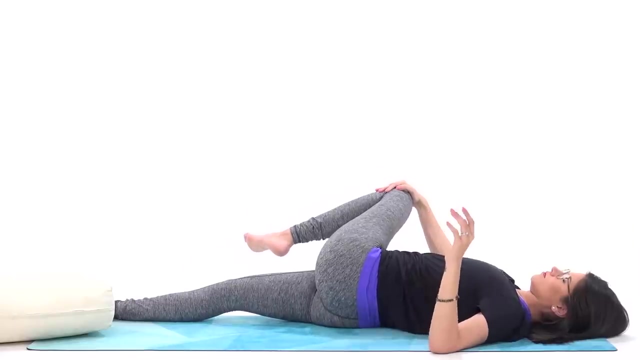 taking a moment to reset. Relax. Then, when you're ready, take your time as you switch sides. Right leg goes long Down on your mat. Slowly and gently draw your left knee across your body, finding your variation of your supine spinal twist. 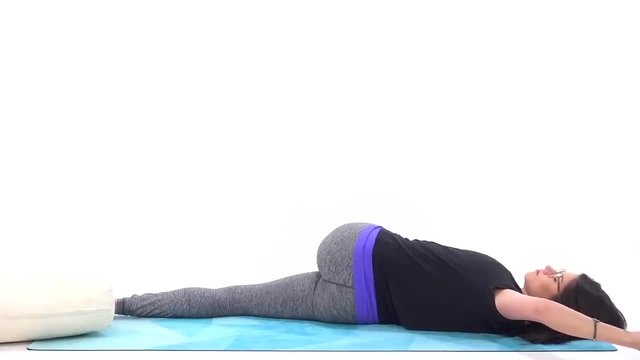 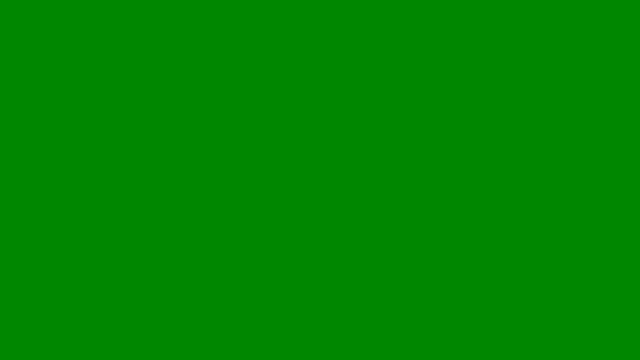 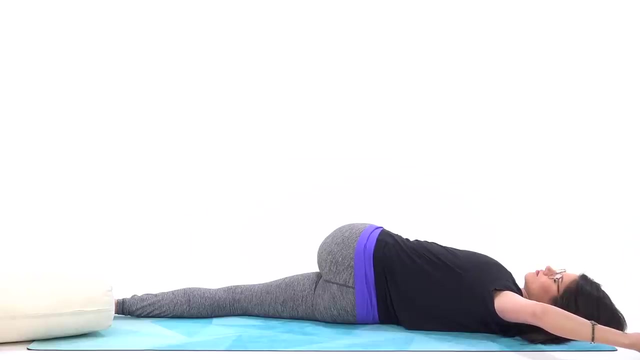 Go for a deep Bryan's or Axial Glute. Relax Laun Malakana. Repeat 1 exercise today. Why do we exercise this? ***? naesan k'omalildis ***, ***, ***, ***, ***, ***, ***, ***, ***, *** ***. 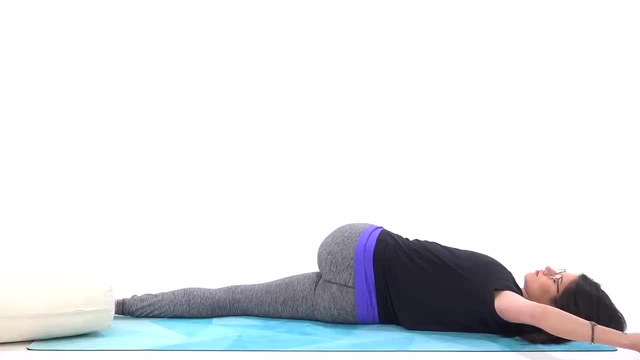 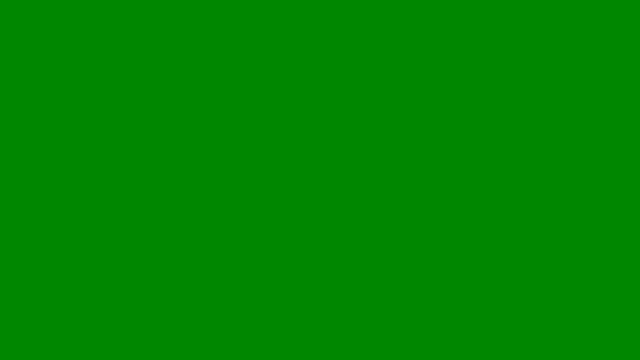 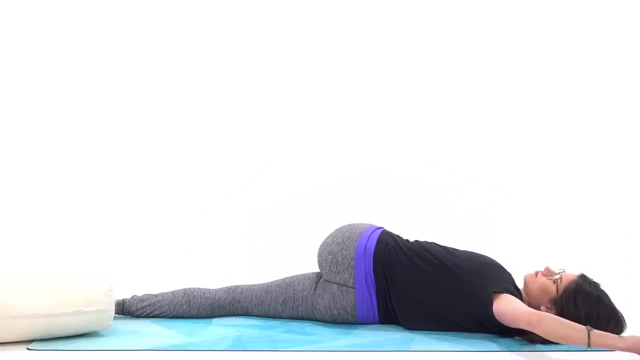 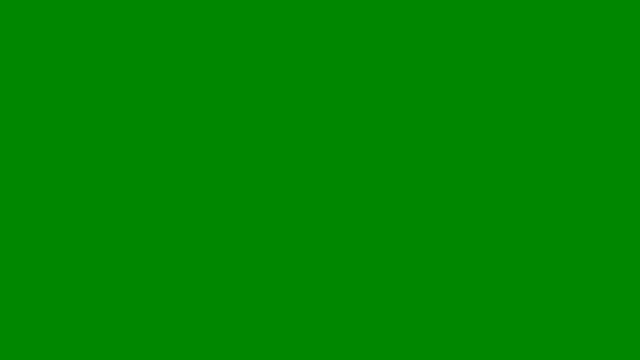 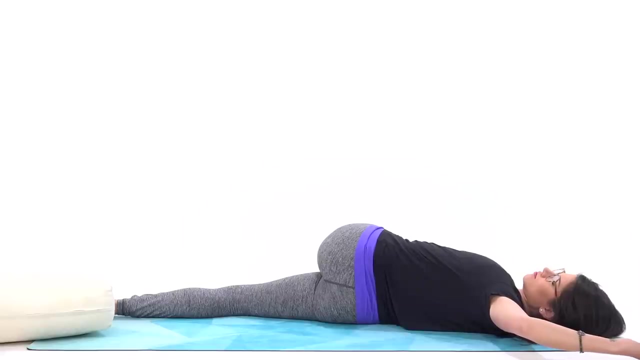 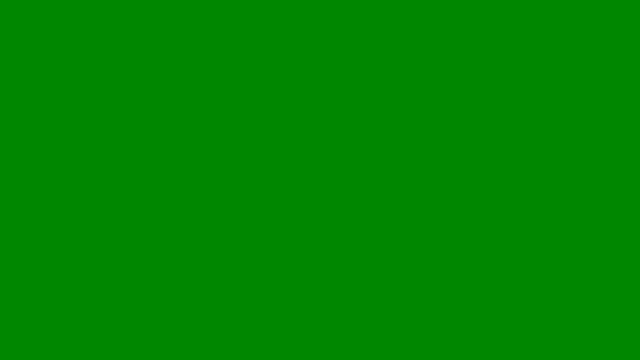 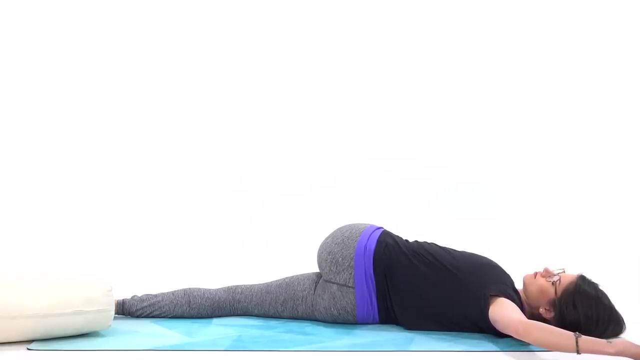 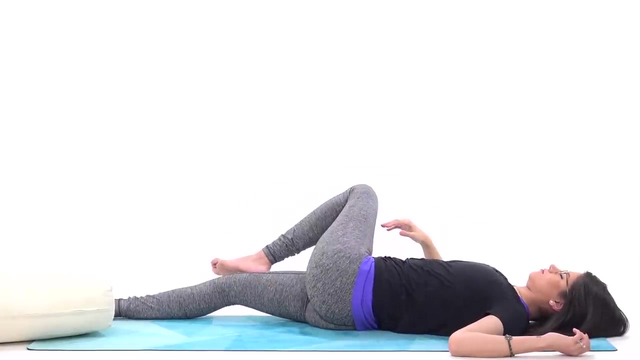 *** *** *** *** ***. Notice how your breath naturally lengthens your torso on your inhales and relaxes you into place on your exhales. Thank you, Thank you, Thank you, Moving slow undo your twist, drawing both knees back into your chest. 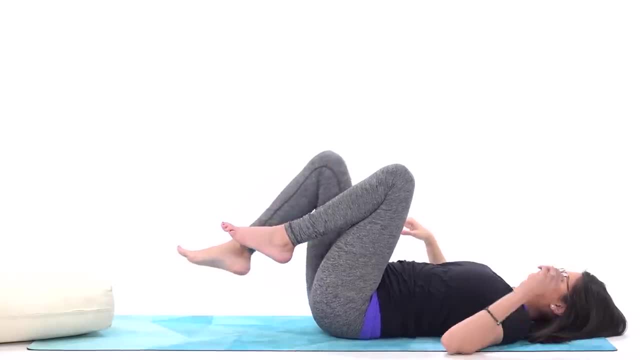 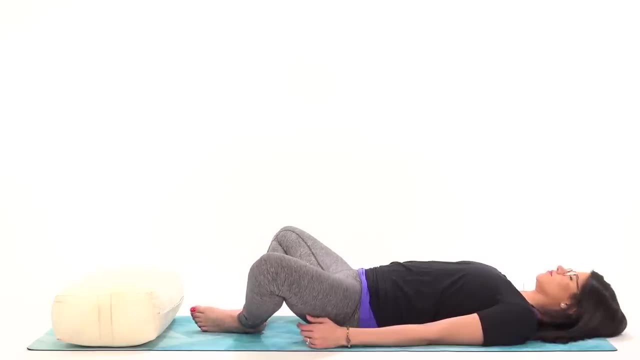 For Supta Baddha Konasana. bring the soles of your feet together, allow your knees to fall open And, to start, you can rest your hands on your belly or take your arms overhead, fingertips touching, and let your elbows fall open. 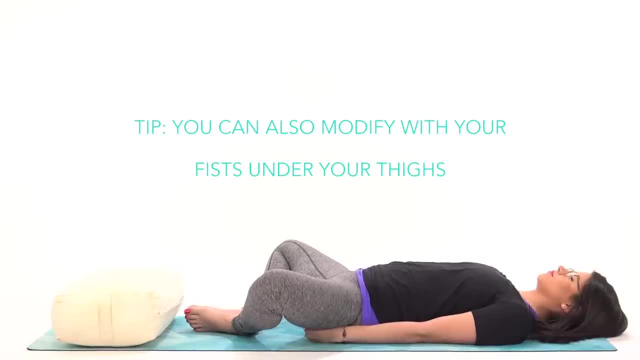 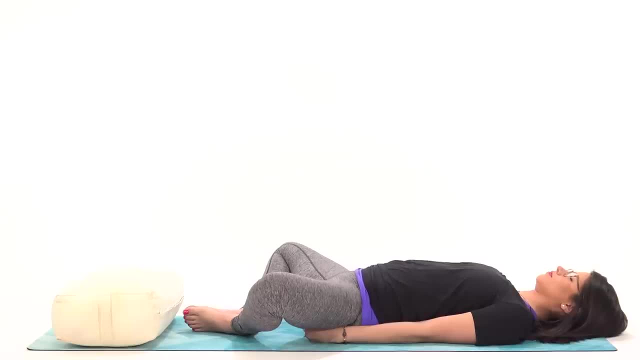 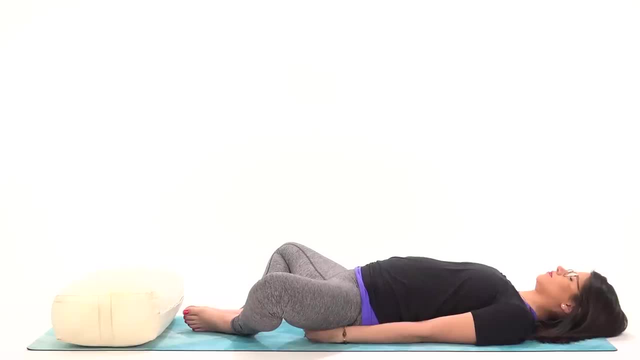 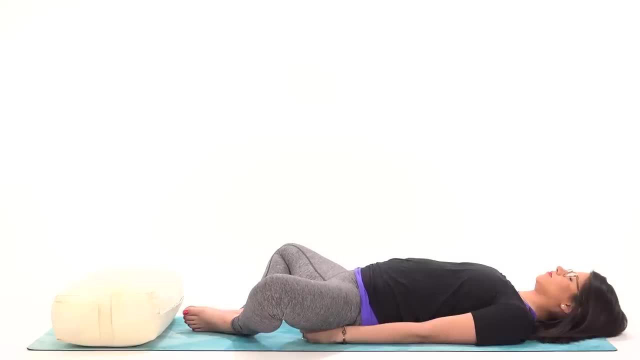 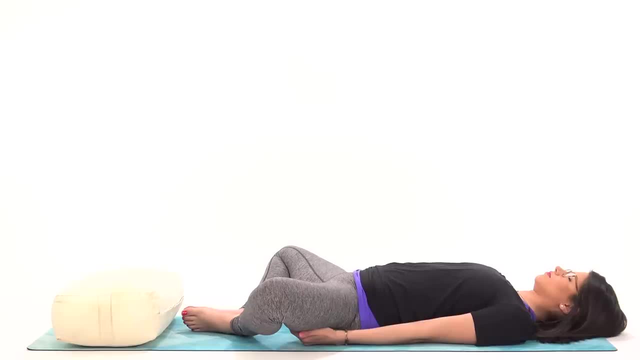 the muscles in your face. I hope you have a wonderful day and I'll see you in my next video. Take care, Bye-bye. Slowly bring your hands to your thighs and assist your knees together and into your chest for a full wind pose. 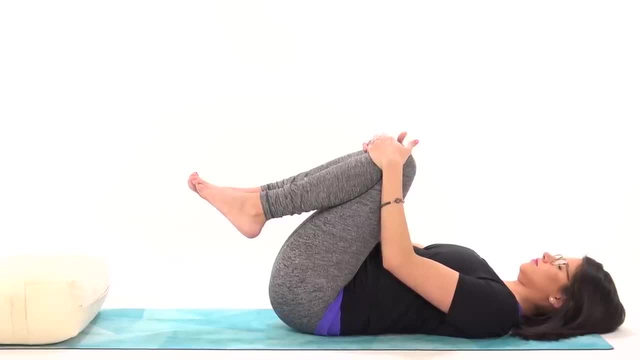 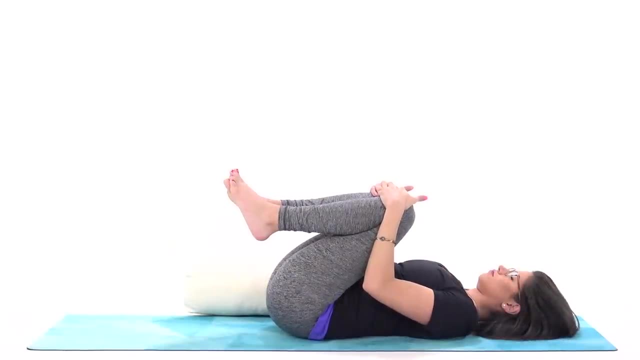 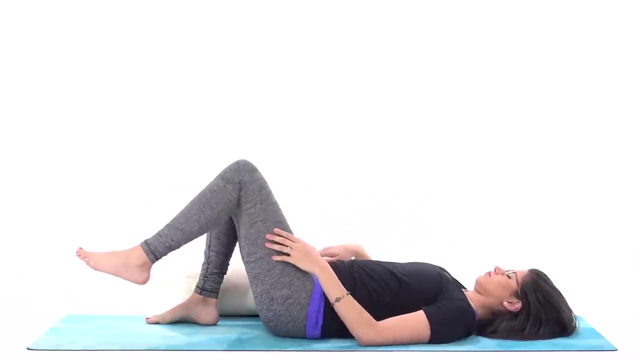 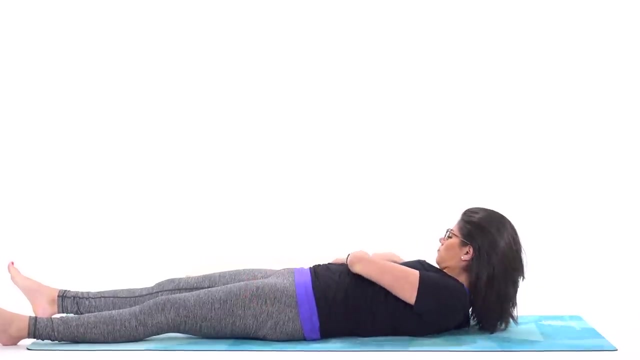 And, when you're ready, release your legs for your final shavasana, Taking your legs a little wider than hip distance. let your feet fall open, with your arms down by your sides, but maybe a little wider than your mat, with your palms facing. 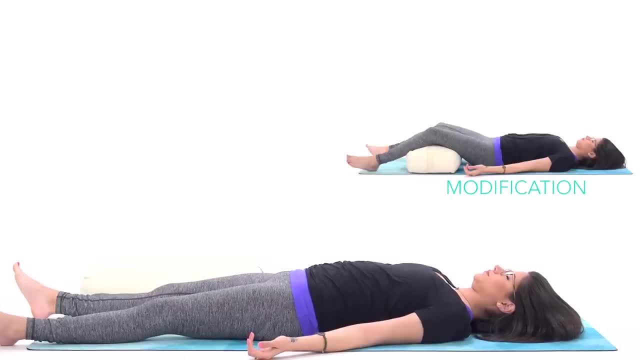 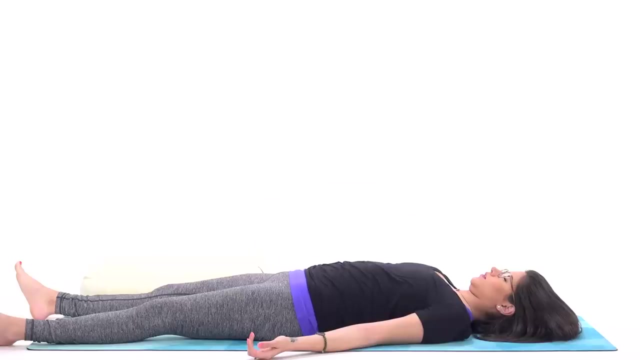 up, Relax your shoulders, Relax your hands, Relax your shoulders. Feel free to inch the back of your head away from your shoulders, lengthening the back of your neck and soften your jaw. Close your eyes and soften the muscles across your face, your eyebrows, your eyelids and. 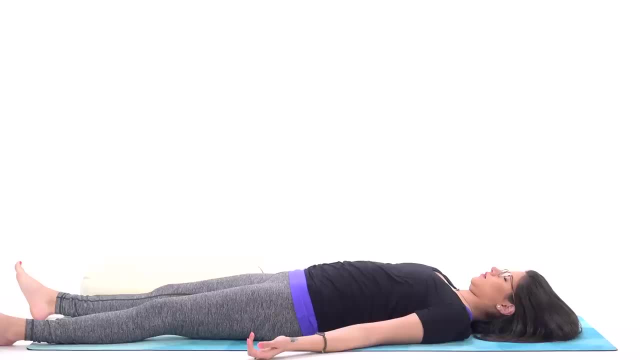 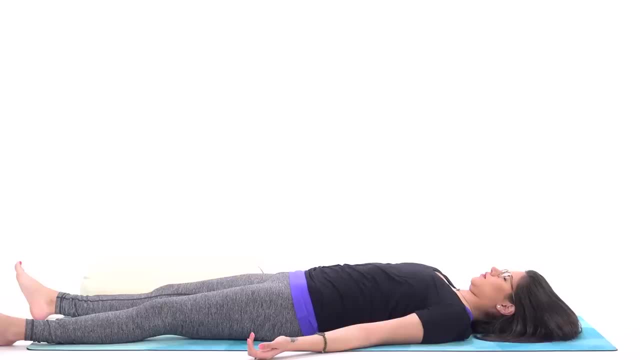 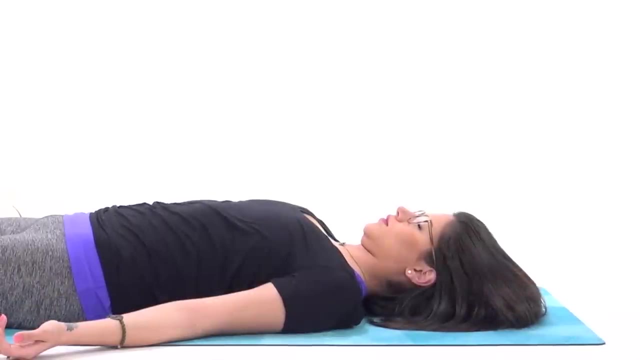 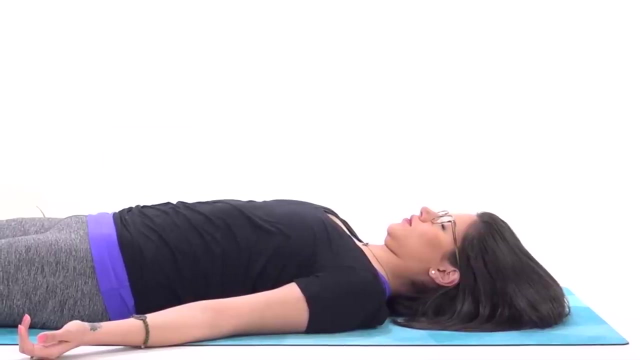 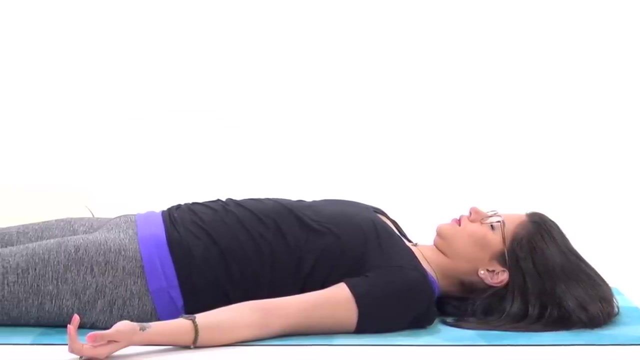 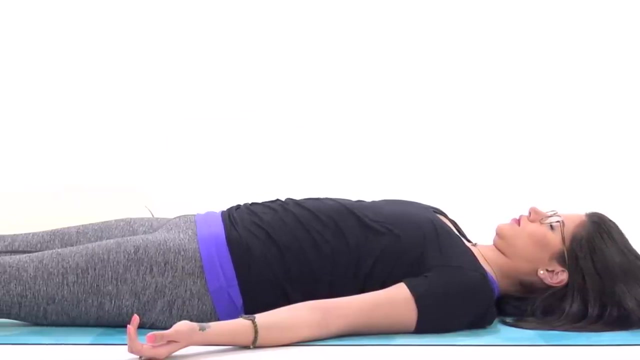 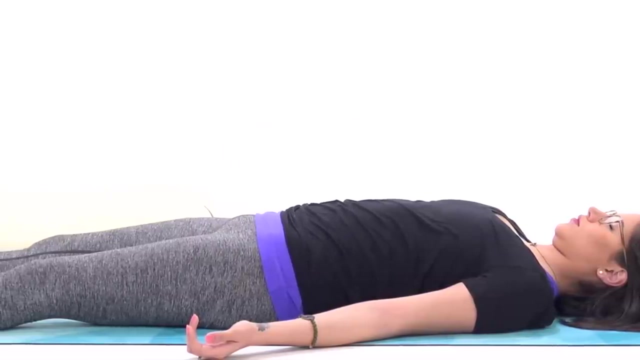 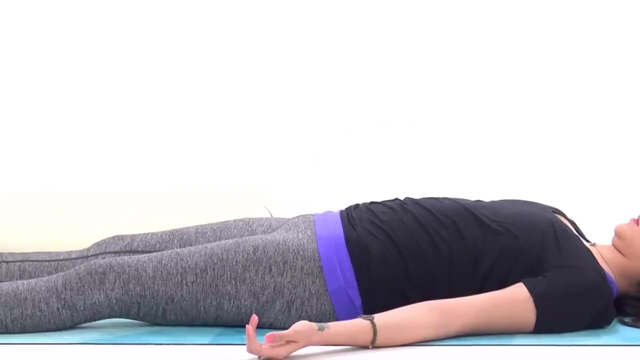 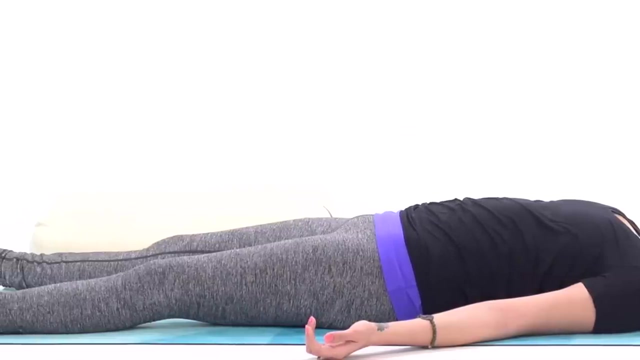 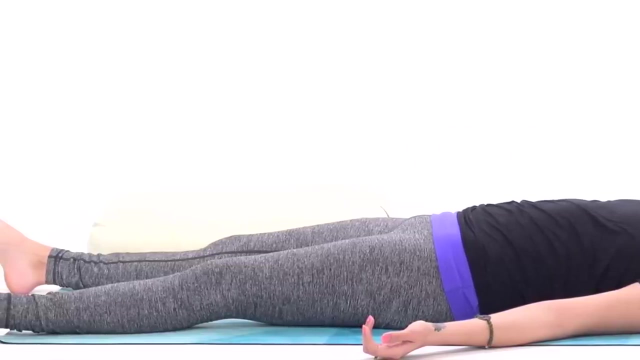 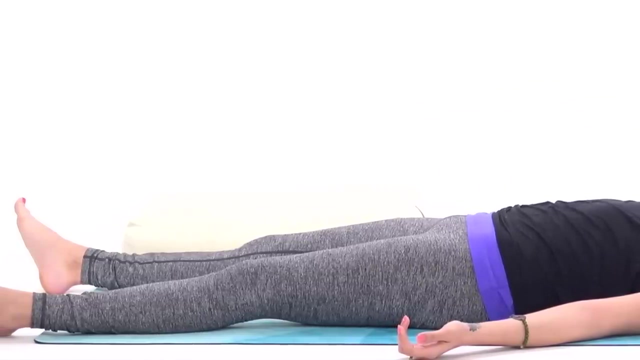 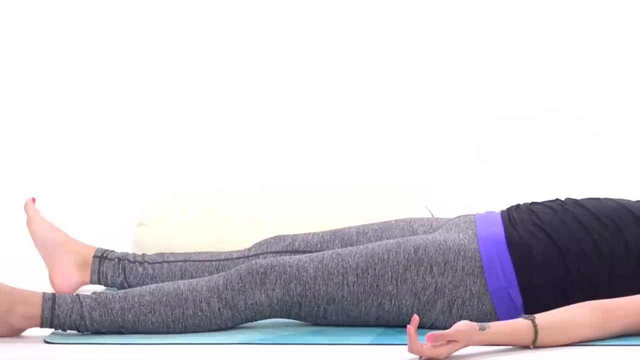 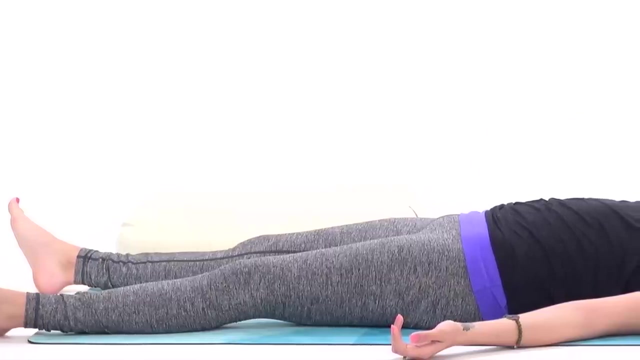 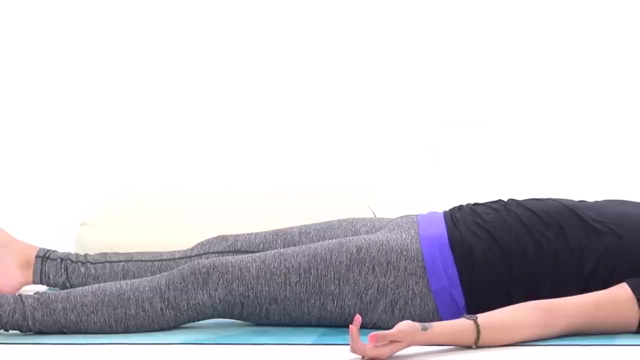 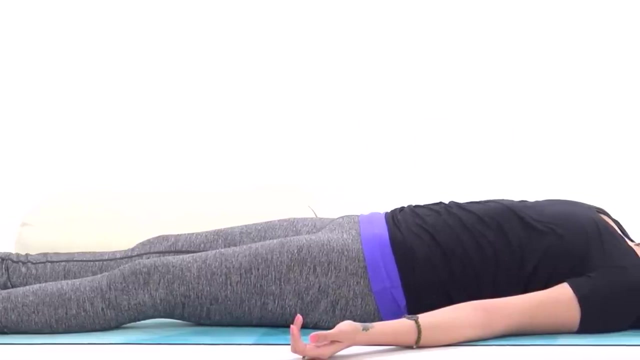 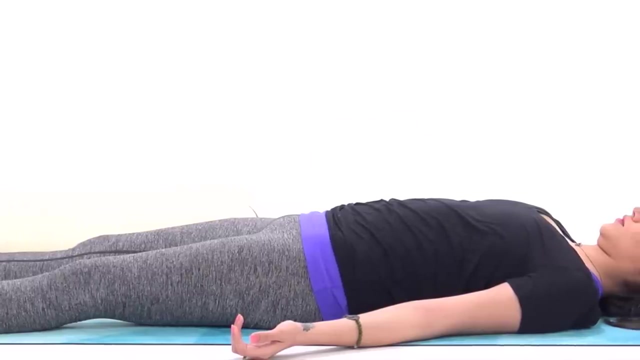 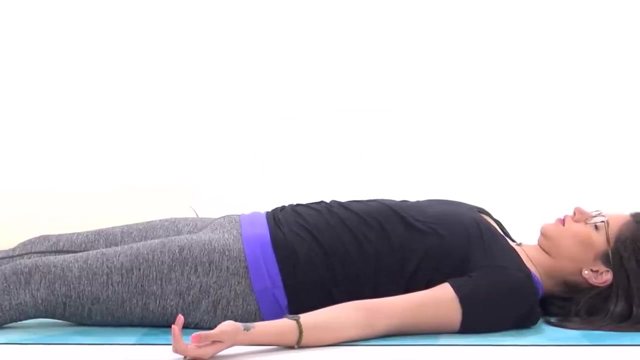 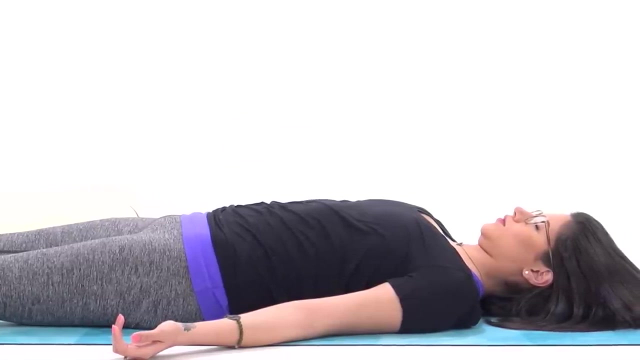 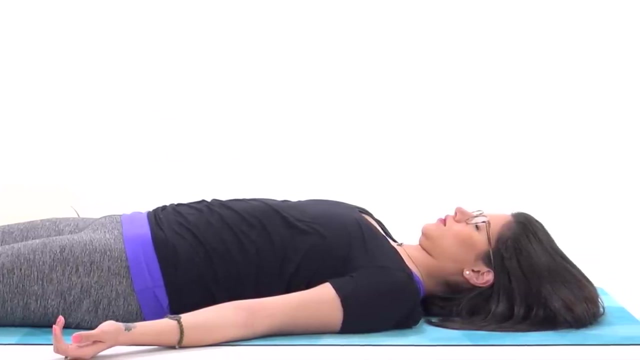 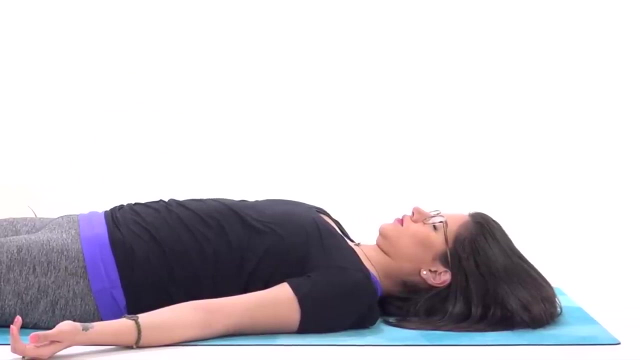 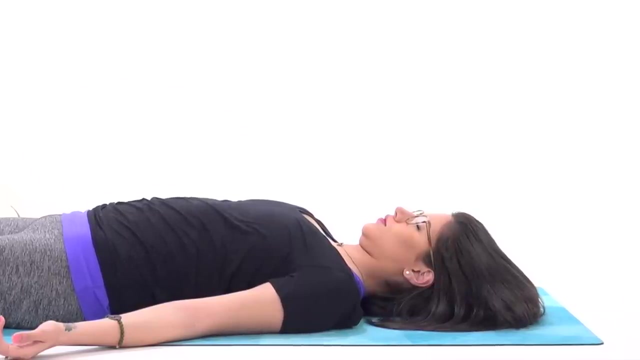 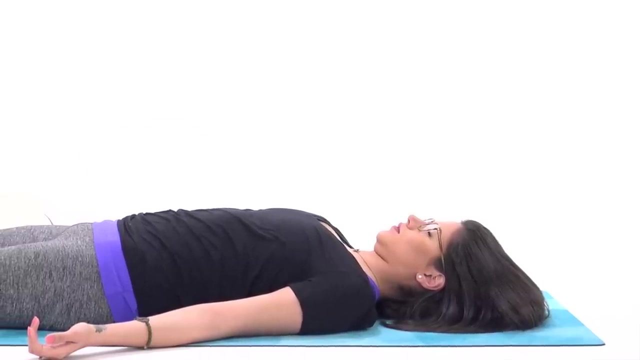 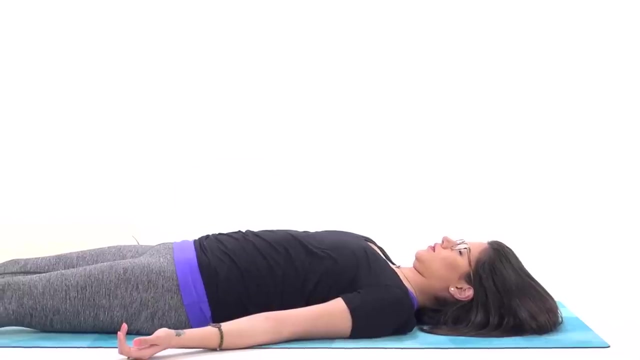 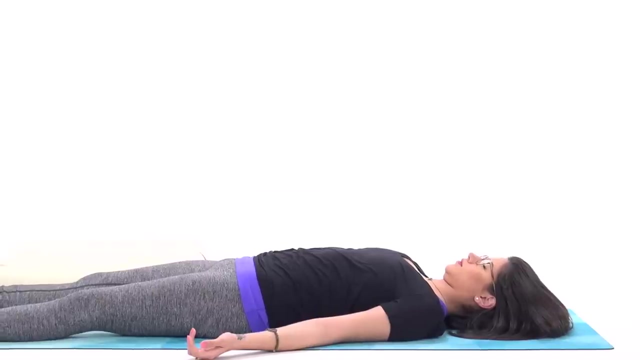 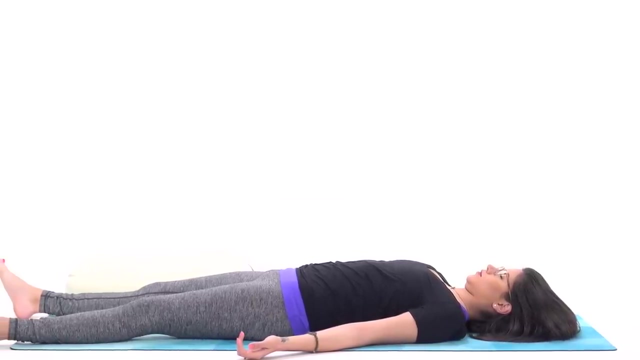 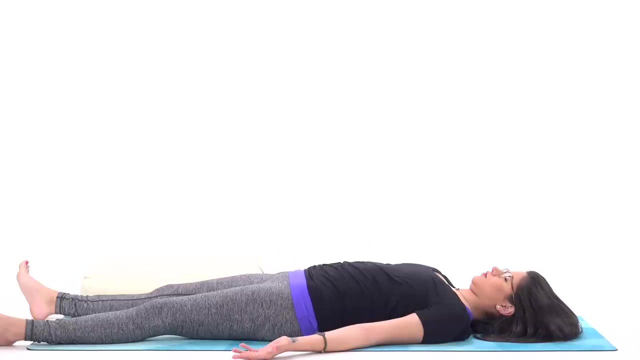 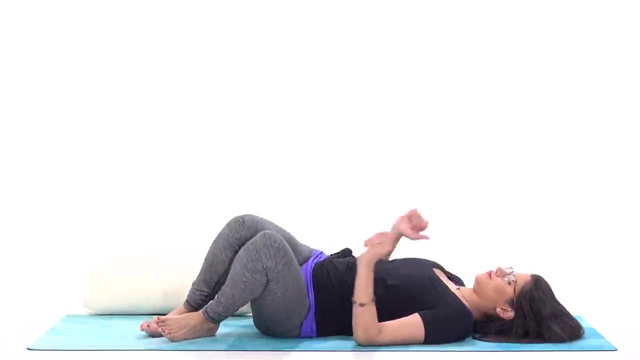